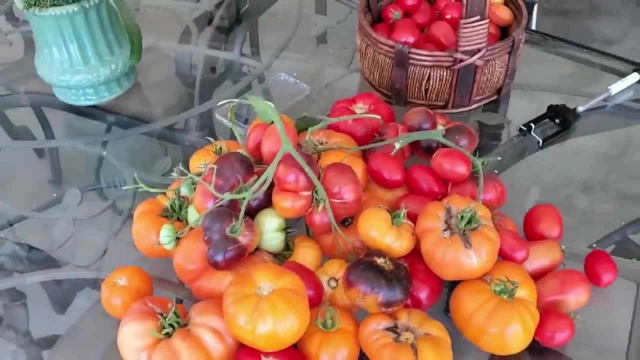 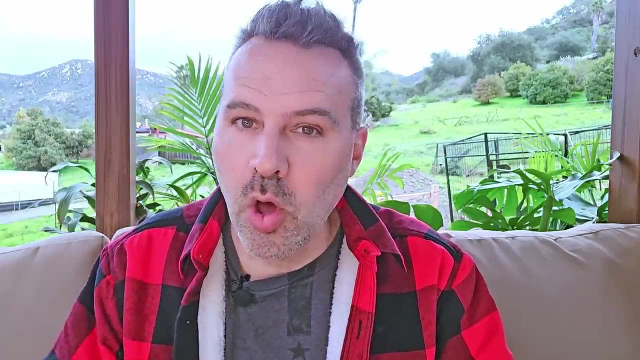 reason. There's absolutely no comparison in taste between a store-bought tomato and a homegrown tomato. By the way, for all the choices in this video, I have video growing guides and I'm going to link them all down in the description box If you're interested in learning more about. 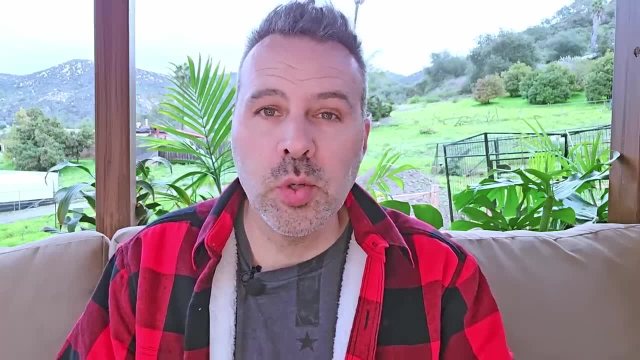 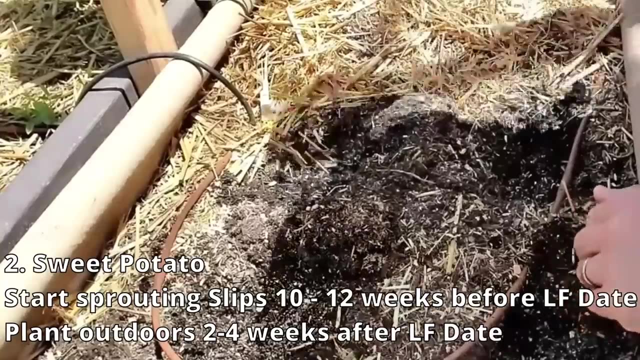 how to grow tomatoes. you can find them all down below in the video description, so you'll have all the info you need to grow all of these choices successfully. My second choice is sweet potatoes. Contrary to popular belief, sweet potatoes and potatoes aren't related. Sweet potatoes are 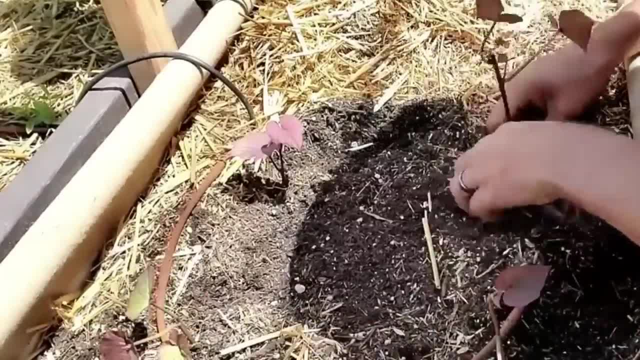 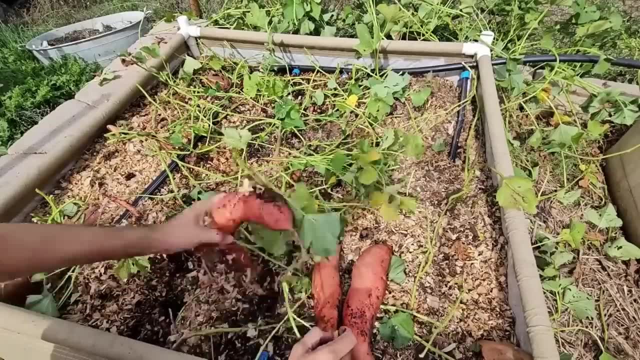 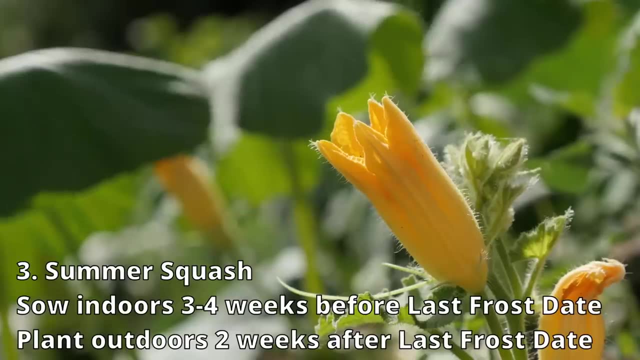 related to the morning glory and potatoes are in the nightshade family. Sweet potato vines do spread and take up a lot of space, but they can also be grown in large containers. Number three is summer squash. Squashes and melons are fun crops to grow. 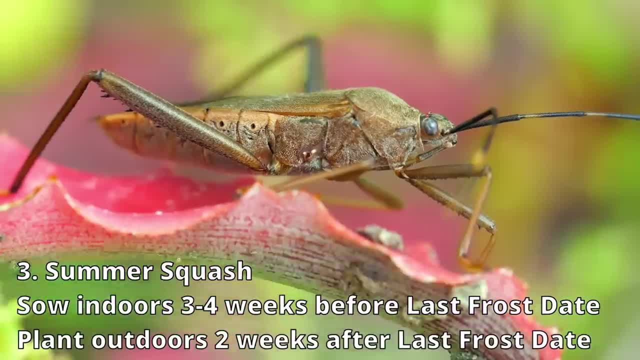 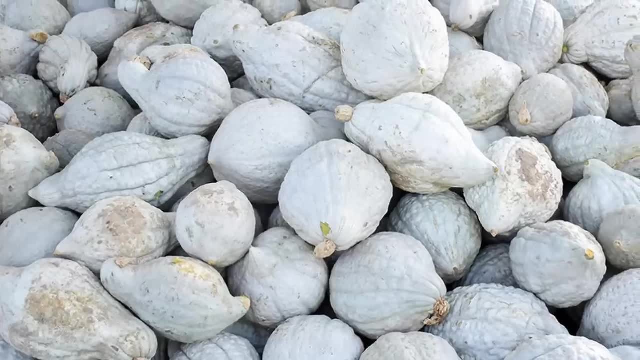 And super easy to grow. unless you're in an area frequented by squash bugs or vine borers, You know they can devastate an entire crop seemingly overnight. Studies have shown that squash, vine borers and squash bugs prefer blue hubbard squash over all others. Plant a trap crop. 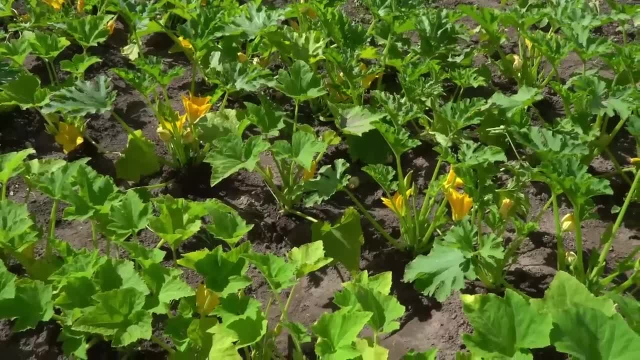 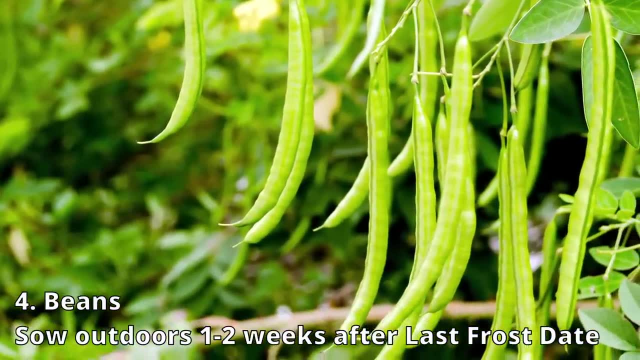 of blue hubbards a month earlier than your main crop. to give them a head start, They should be 10 to 15 feet away from the crop you're trying to protect. Number four is beans. There are two types of beans: Bush and runner. And how do you know which one is which If you're looking for a good 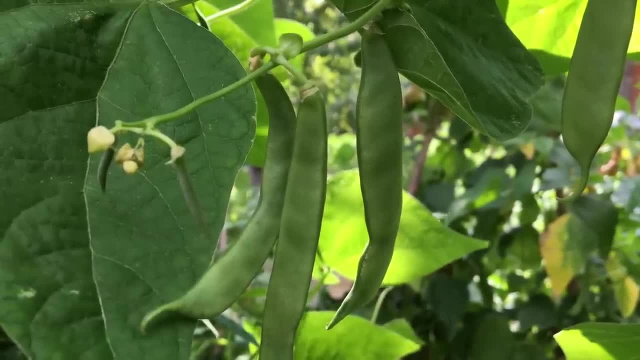 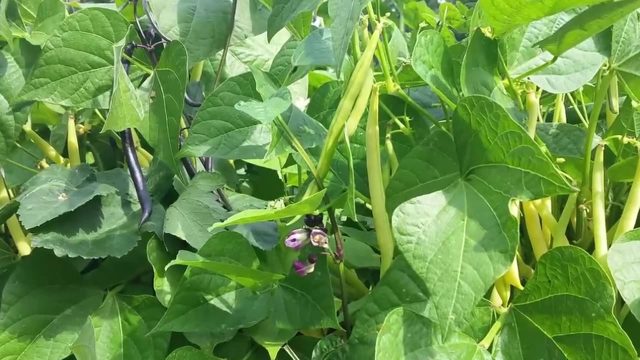 bean. you can grow beans in your garden, no matter what size or shape it might be. You'll need to grow runner beans on a trellis of some kind. Bush beans are very prolific, though, and you won't need a trellis for those. You can even grow them in a container. Number five is 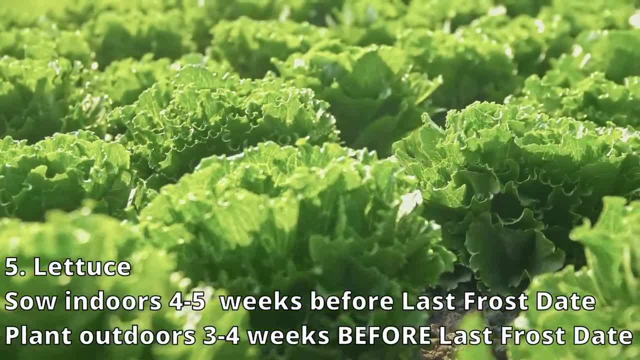 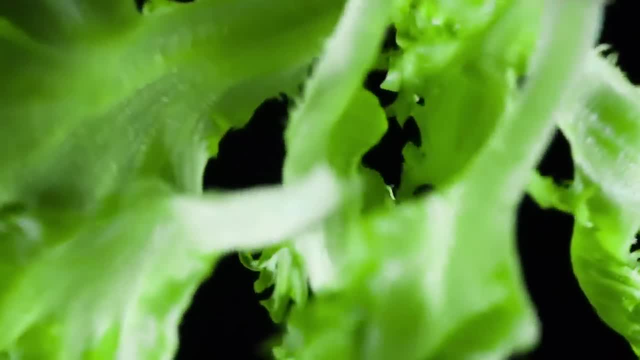 lettuce If you've never gardened before. lettuce is a great starter plant, especially leaf lettuce. It germinates and grows quickly and you can start harvesting in less than a month. There are two main types of lettuce: Leaf lettuce and head lettuce. Head lettuce takes more space. 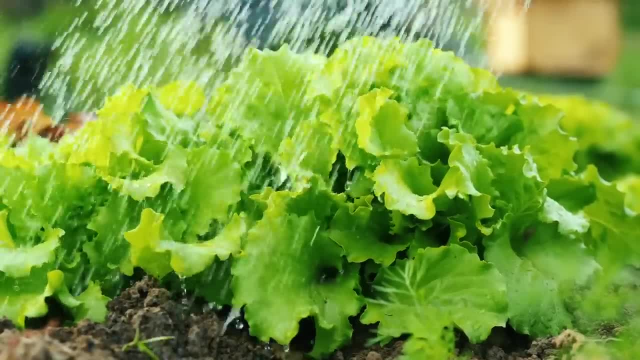 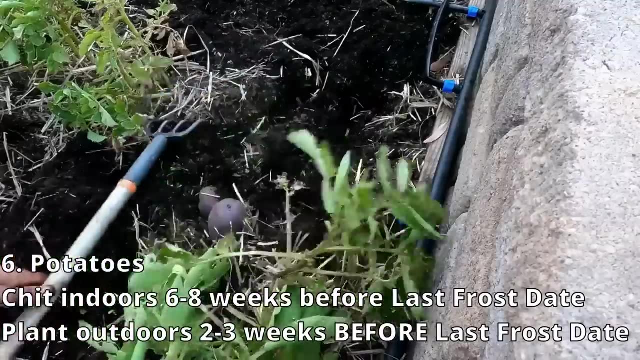 and takes more time to grow, while leaf lettuce is quick growing and can be tucked in just about anywhere. Number six are potatoes. Potatoes are one of the most fun things to grow and you never know what you're going to dig up at harvest. Aside from the fun of growing them, the flavor. 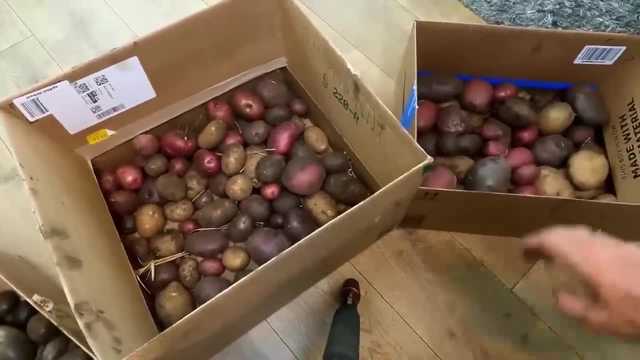 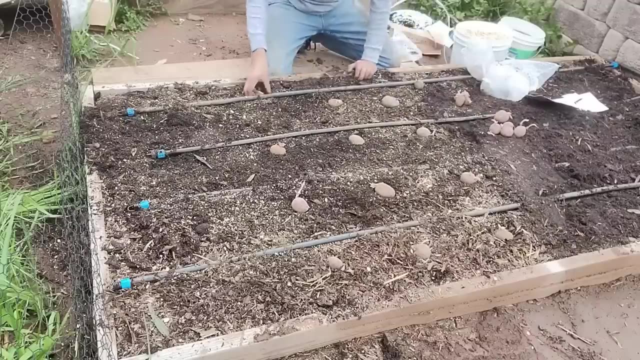 of homegrown potatoes fresh out of the earth is way different than you might think. Remember to check the links in the video of this description, because I have a video on how easy it is to grow potatoes without ever digging to plant them or digging to harvest them. 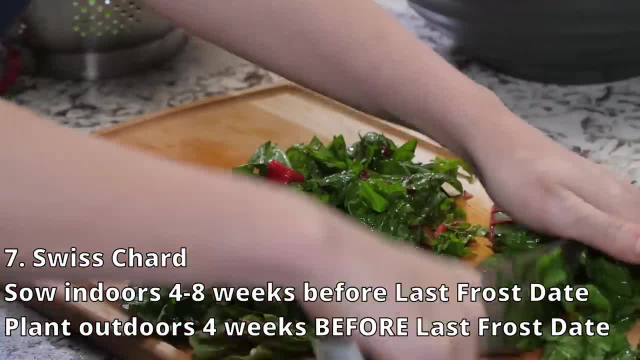 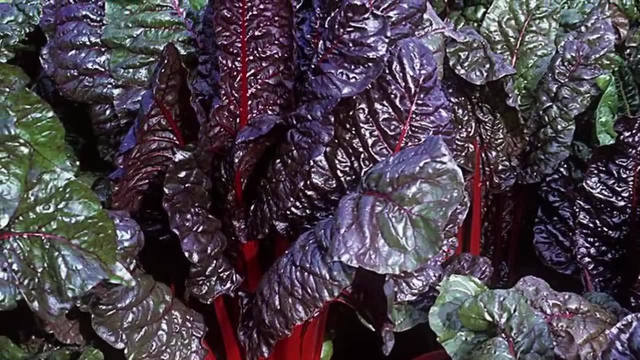 Number seven is chard. Both the stems and leaves of chard can be eaten, cooked or raw. Swiss chard grows to a large size, so leave plenty of room in the garden bed. You probably only need one or two plants. Chard is extremely cold, hardy, down to 15 degrees Fahrenheit or negative 9.4. 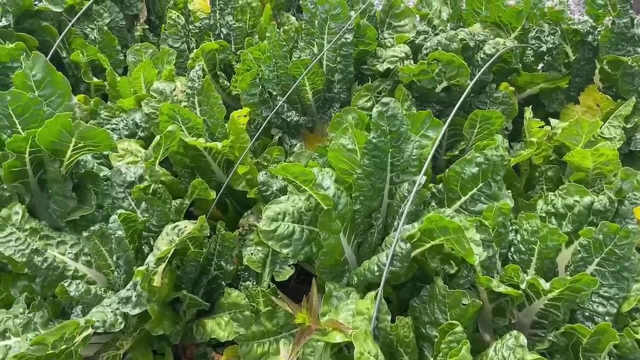 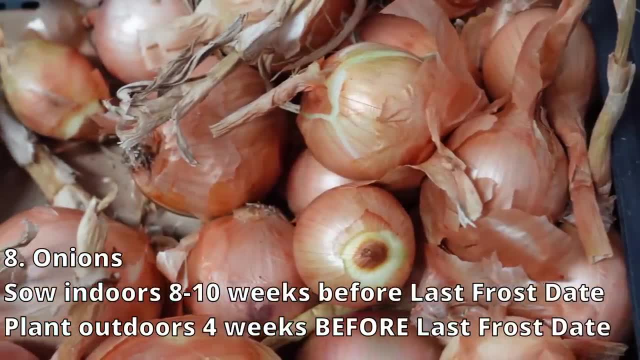 Celsius. On the other hand, it's also heat tolerant, much more so than lettuce, so you can continue to harvest chard through the summer to use in salads. Great is onions. Onions have been in cultivation for thousands of years. I can't think of many of my favorite recipes that don't include onions. 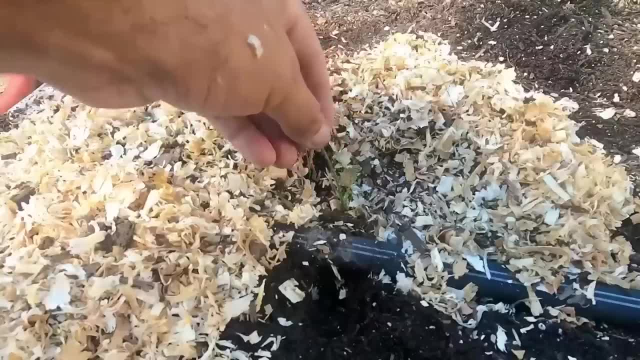 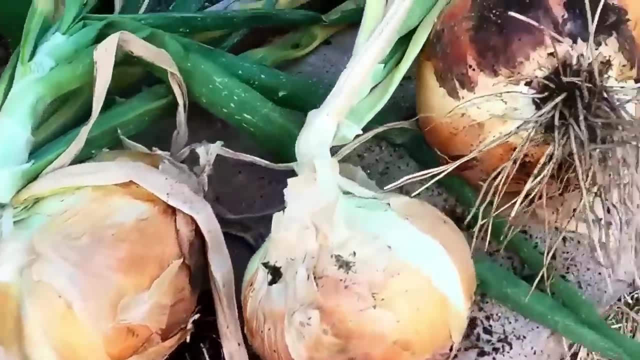 I find growing my own and cooking with them to be so satisfying. They're delicious and add so much flavor to so many dishes. They take up very little space when interplanted with other vegetables and they're easy to grow when you follow a few basic rules. Now, the last two are plant families. 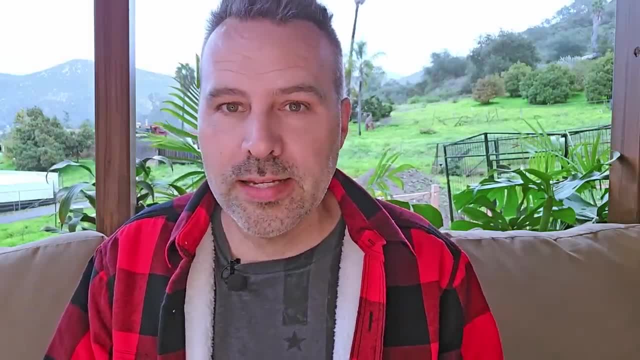 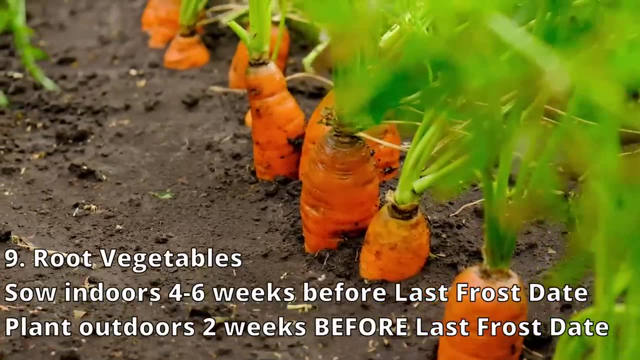 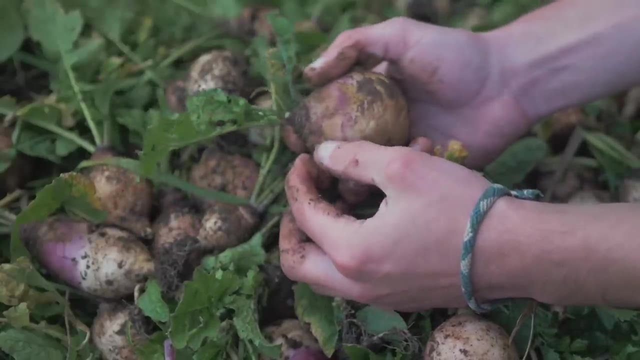 or plant groups that can be grown really well when planted right now. Nine is root veggies like chard. Chard can be grown in any weather except freezes. That means they're some of the first planted in any garden In mild winter climates. these make up the bulk of our fall, winter and 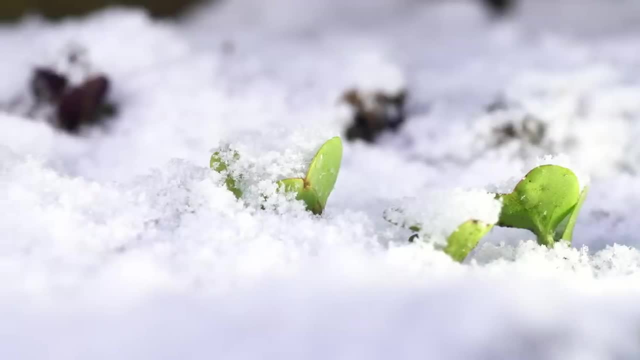 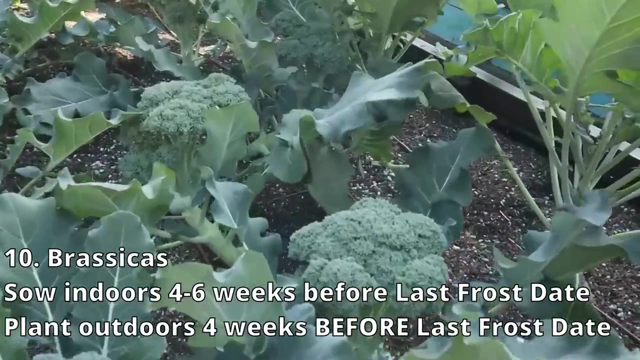 early spring garden, but can also be grown through the heat of summer In cold winter climates. these are usually planted or sown in late winter, early spring, and grown through until your first freeze. Number 10 is brassicas. This is a family that includes broccoli, cauliflower, Chinese cabbage. 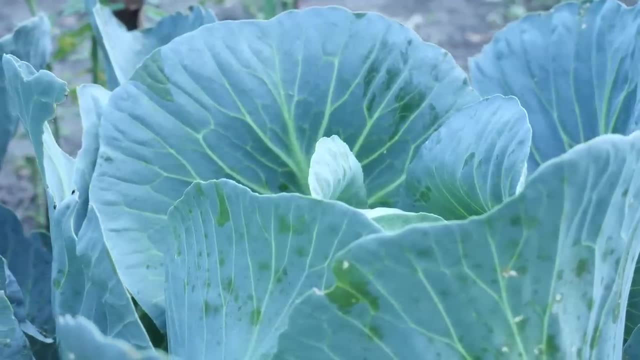 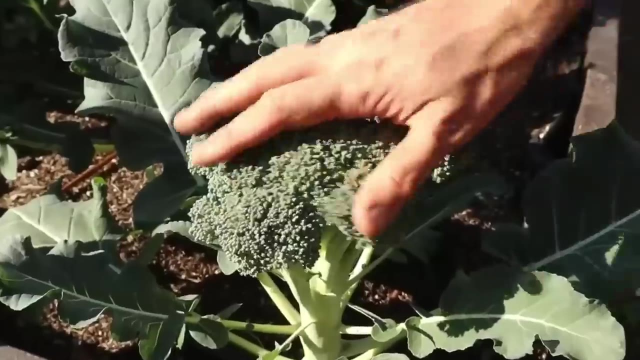 regular, cabbage, kale, kohlrabi. these amazing plants are known to survive freezes down to 25 degrees fahrenheit or minus 3.8 celsius. Most are long growers, meaning they take months to mature. These are great options for space. 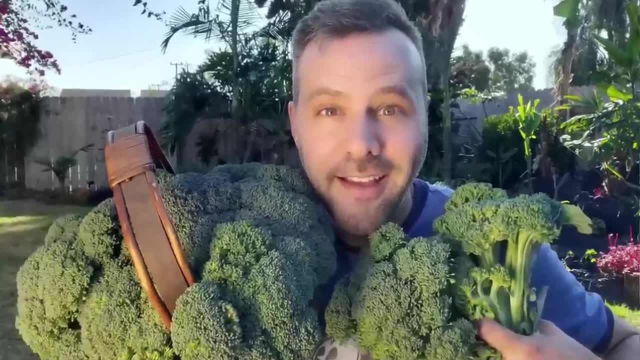 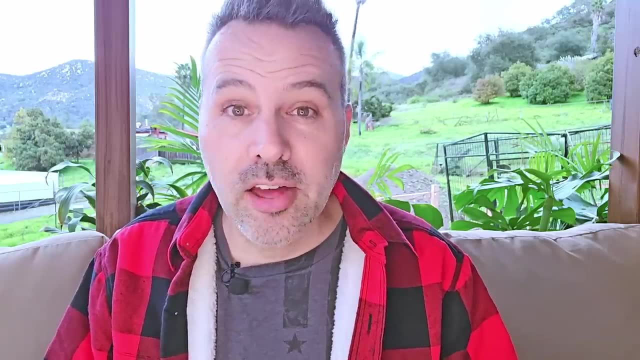 saving interplanting, Because they take so long to grow to harvest. you can plant quick growing crops right around them to maximize space. That's my 10 choices, so get busy right now to make 2024 your best garden year ever. If you're getting ready to start seeds, watch this video right here, so you